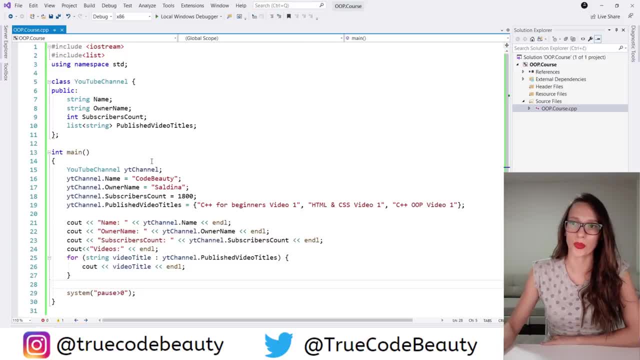 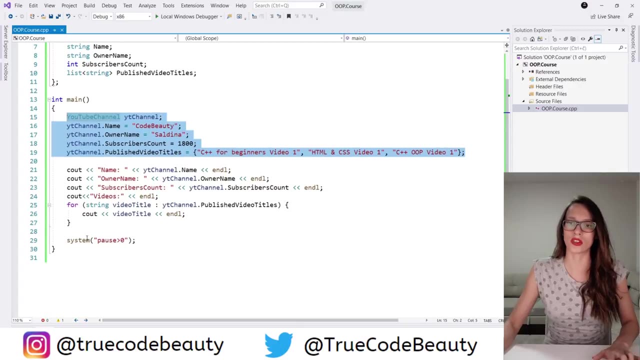 you can really understand the need for these two. So what happens? if I want to create another object of this YouTube channel class? I'm going to do that. Well, in this current situation, what I would do is I would copy this, So I'm going to copy it, and then I'm going to. 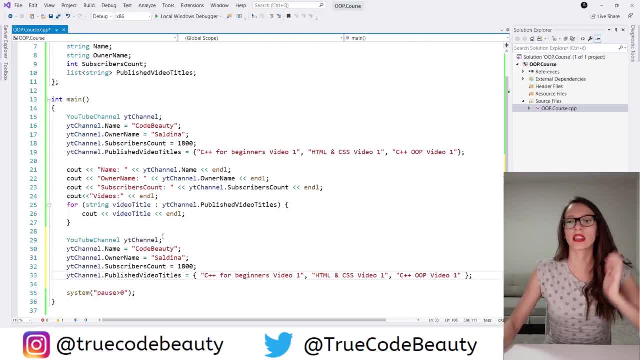 paste it here like this And let's give it a name. Let's say that this channel is going to be YouTube Channel 2. And let's call it. let's say: YouTube Channel 2.name. Let's say that it is going to be called. 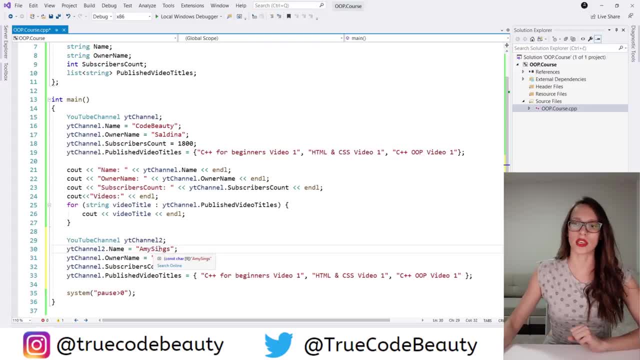 Amy Sinks, for example, And owner is going to be a girl called Amy, and then she is going to have, let's say, 2,000 subscribers. okay, and then the videos that she has published are going to be songs. 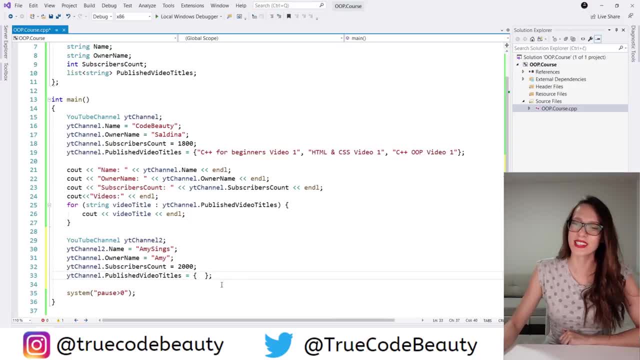 obviously, because she has a channel named Amy Sings. so let's say that she has published, for example, let's say, Johnny B cover like this: so that's one song, that's one video. and then let's say that another video that she has published is going to be, for example, 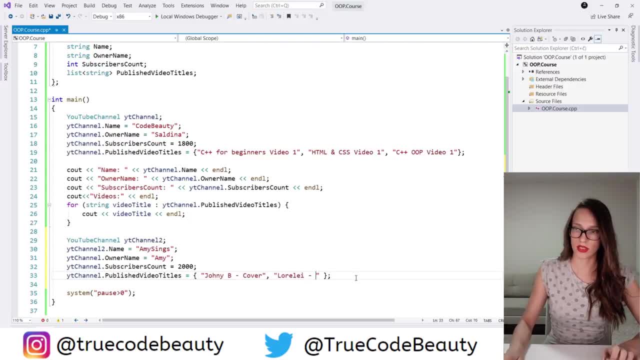 Lorelai, so that's a song from Scorpions and she has made a cover of that song like this. now, these two are two of my favorite songs and you can put whatever you want here in this list. and I'm also wondering, and you can write that in the? 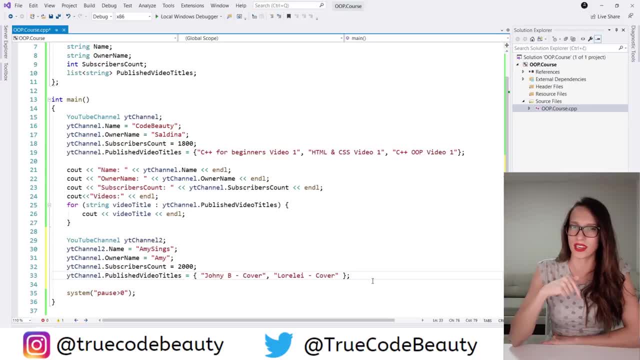 comments down below what are your favorite songs. so please write that in the comments. just don't put links, because I think that YouTube has this policy of treating links as advertising or spam or something. so just write out the name of your song and then the name of. 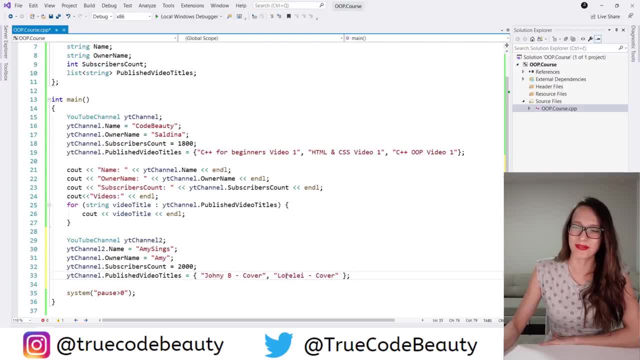 a singer, I guess, and I'm really looking forward to reading your comments. so, now that I have created this second YouTube channel, I'm going to put links to my favorite songs, and I'm going to. what I want to do is I want to write out information about this channel, but I noticed 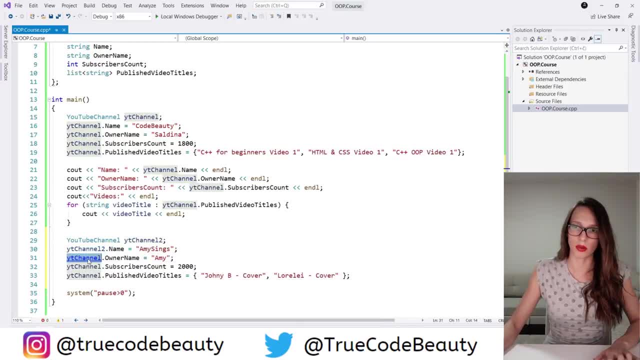 that I'm missing here, this YouTube channel 2, so here I'm going to say: YouTube channel 2.owner name, and then YouTube channel 2.subscribers count, and then YouTube channel 2.published video titles as well. okay, now, if I wanted to write out information about this second channel. 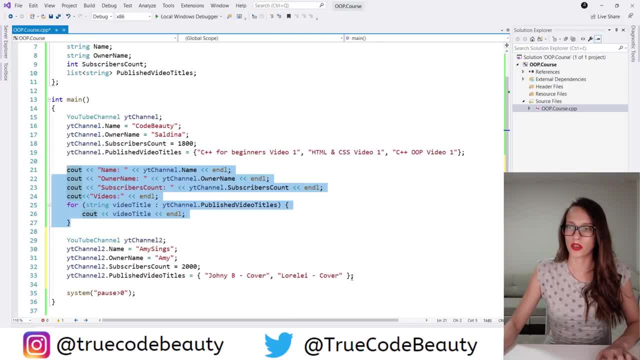 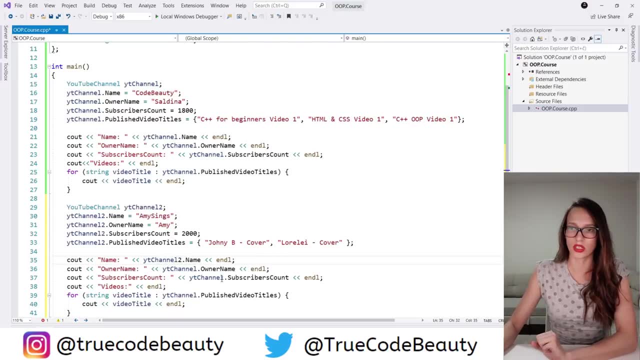 what I would do is I would copy this. so I'm going to copy it and then paste it here and here I will say that the name is YouTube channel 2.name, and then owner name is YouTube channel, 2.owner name, and then here as well, and then YouTube channel, 2.published video titles. 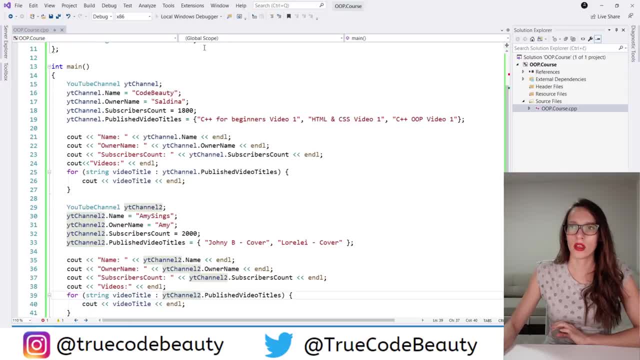 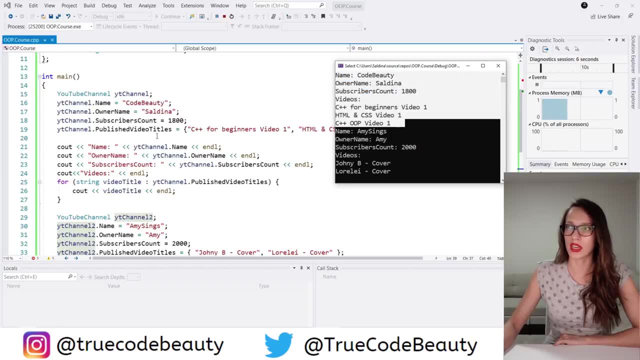 okay, now, if I run this program, we should get information about these two channels. so the first channel is this one that we already had it's Code Beauty owner is me, and then this is subscribers, and then these are three videos that I published so far. I mean, I published more than three videos. 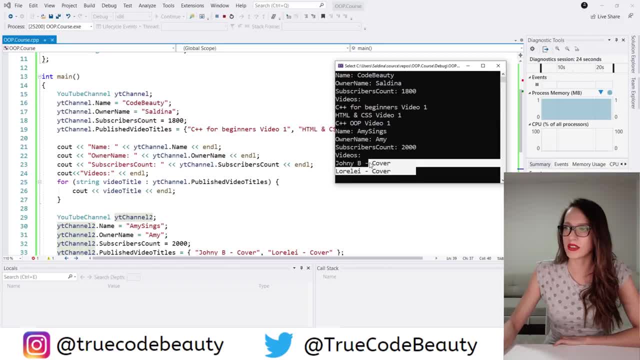 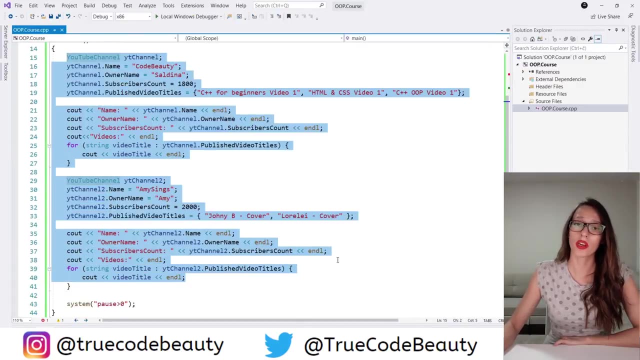 but this is just an example. and then here is our second channel. it's called Amy Sings and then owner is Amy. she has 2,000 subscribers and then she has published two covers. now this here has a problem. if we wanted to create a third, a fourth, a fifth object, we would have to copy. 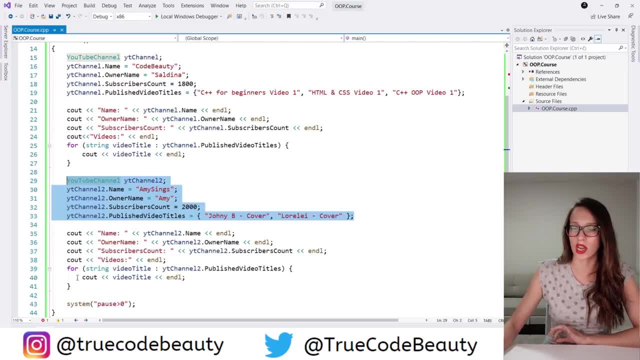 this code and then each time that we want to write out information about those channels, we would have to copy this code. and this really collides with a principle called don't repeat yourself, meaning, do not repeat your code if you don't really have to repeat it. 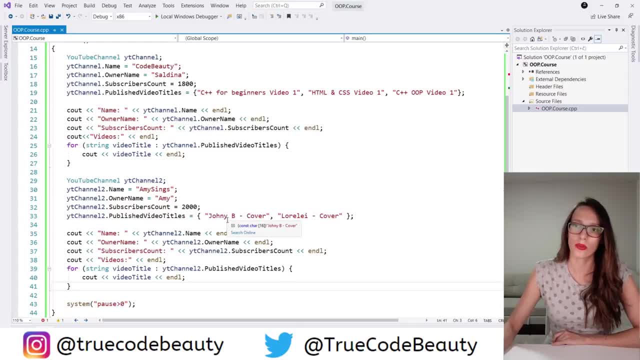 and, in this particular situation, we do not have to repeat it. so how we are going to solve this problem? Well, the first thing that I want to talk about are going to be constructors, and what a constructor is. it is a special method that is going to be invoked. 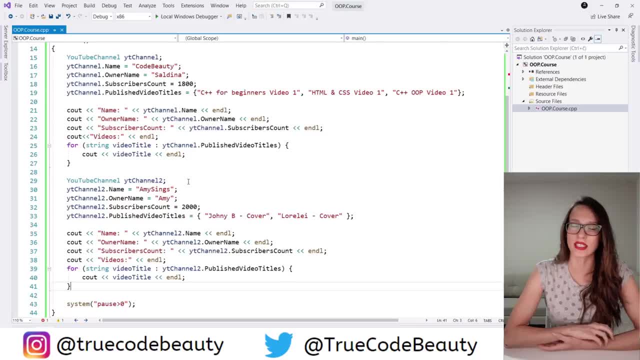 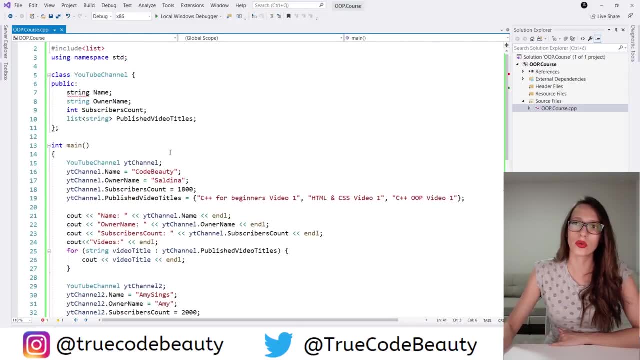 each time that you create an object of a specific class, meaning that method is going to be called on the construction of that object. so there are two rules when it comes to constructors, and the first rule is that constructor has the same name as your class. and then the second rule. 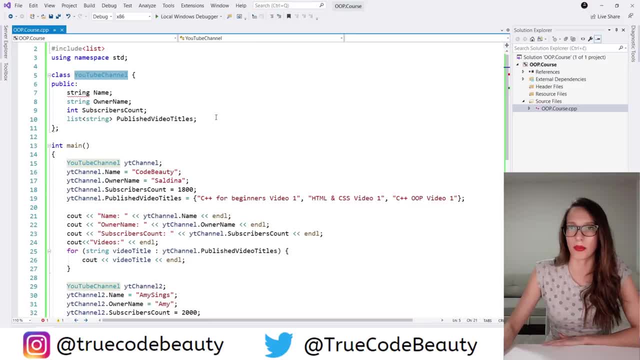 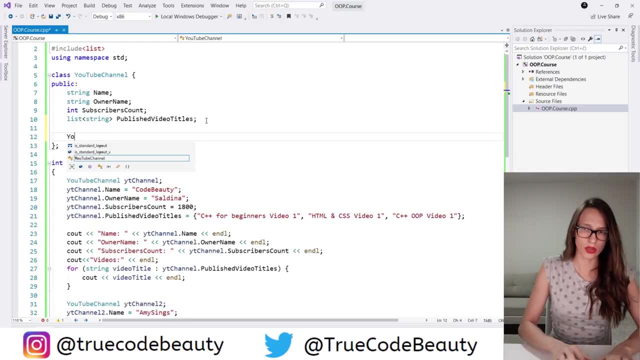 is that constructor does not have a return type. so let's create a constructor for this YouTube channel class Here. I'm going to create a constructor for this YouTube channel class and then I'm going to say YouTube channel like this, and then I'm going to put these parentheses and I'm going to put: 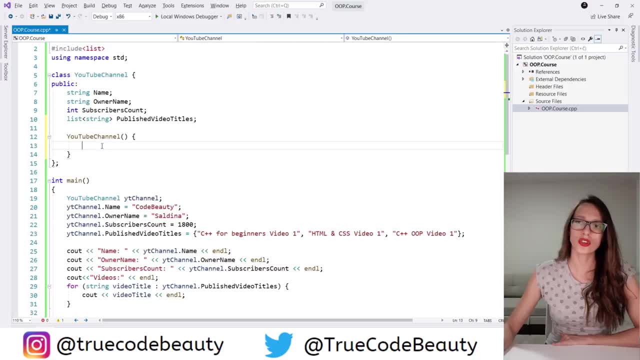 these curly brackets as well. Now, what I want to do in this constructor is: I want to receive two parameters. I want to receive two arguments, and those are going to be string name and then string, let's say, owner name. okay, Now these are two parameters that are going to be used to. 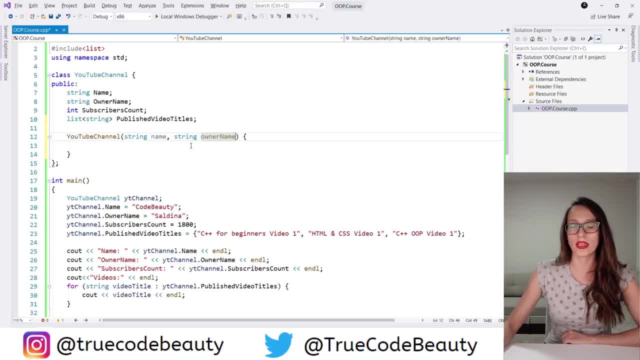 pass to my constructor and what I'm going to do with these in my constructor is I'm going to assign these to these properties here. so I'm going to say that name is going to be equal to whatever my user has passed to this constructor. so name is equal to this name here. and then owner name. 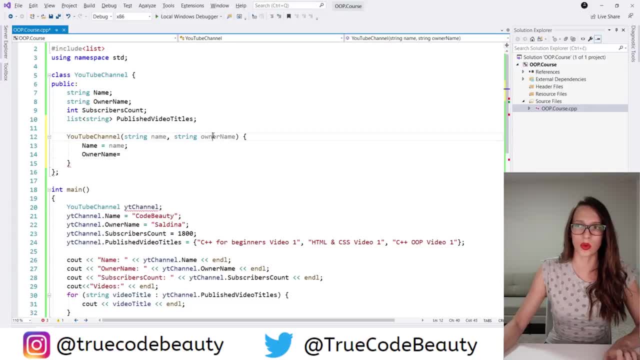 in my class is going to be equal to this owner name that I have received in my constructor. Now, since this constructor is going to be equal to this owner name, I'm going to assign these properties here and then I'm going to say that name is going to be equal to this owner name that I have received. 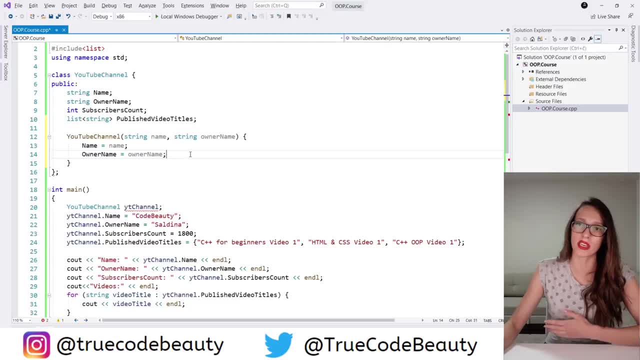 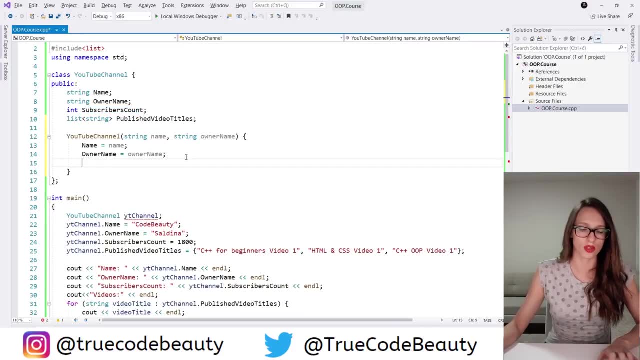 in my constructor. Now, since this constructor here is invoked each time that I create object, each time that it is constructed, that means that at the beginning, when a channel is created, it has zero subscribers. so I'm going to put here zero like this. We do not even have to pass this. 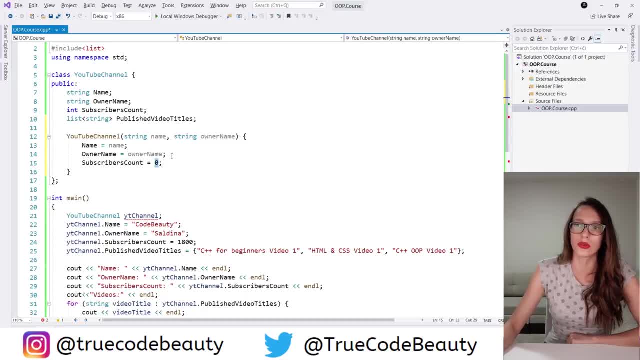 value in our constructor, because when you create your YouTube channel, you do not have subscribers. Okay, now what am I going to do here is, I do not need to write this code like this anymore, so I'm going to delete. I'm going to actually comment this code here and, as you can see, this is underlined. It says that: 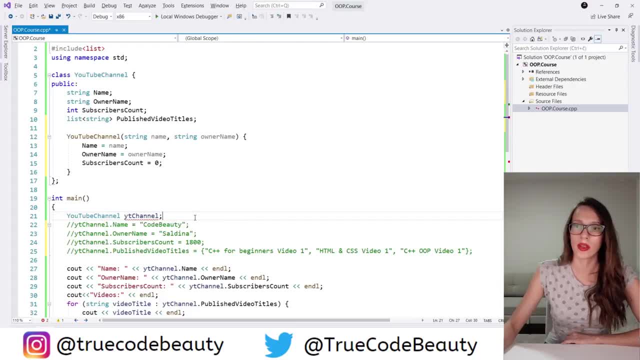 no default constructor exists for class YouTube channel. Now what we have to do is we have to use this constructor here that I have just created. and how you do that? well, you put parentheses here and then, inside these parentheses, we are going to pass these two parameters. So the first: 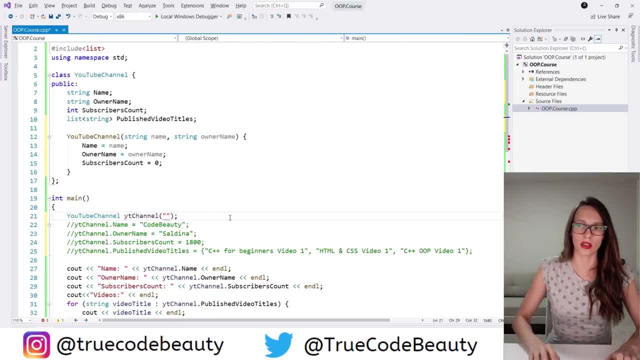 parameter is going to be the name, so that is the name And that is this name here. so code beauty like this. And then a second parameter, as you can see here is owner name and that was this value here. So I'm going to pass that here, like this: 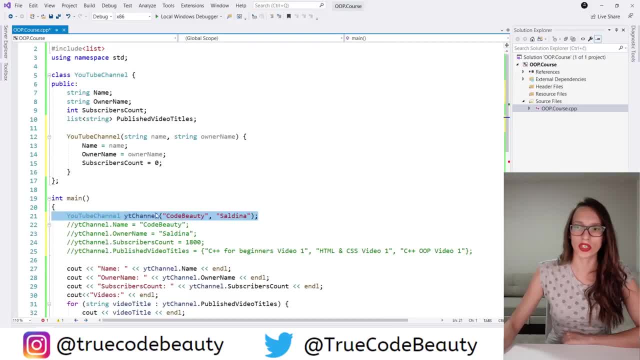 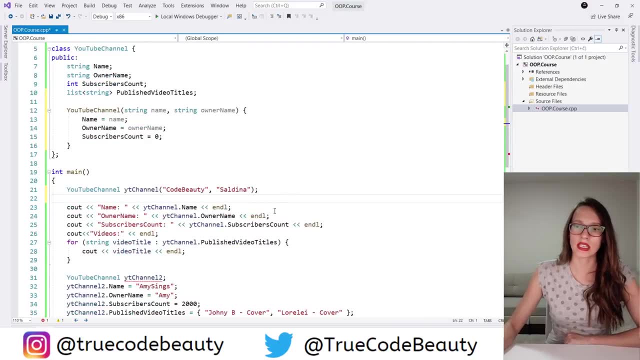 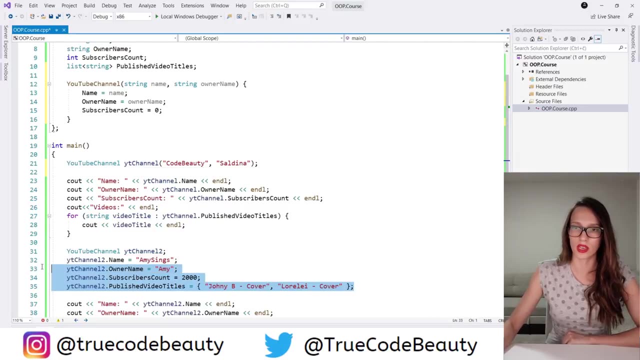 And now, after I have created this YouTube channel, we do not need this code anymore, so I'm going to delete it, Okay, and what we can do is we can do the same with with this second channel, so with this YouTube channel too. So I'm going to really comment this. 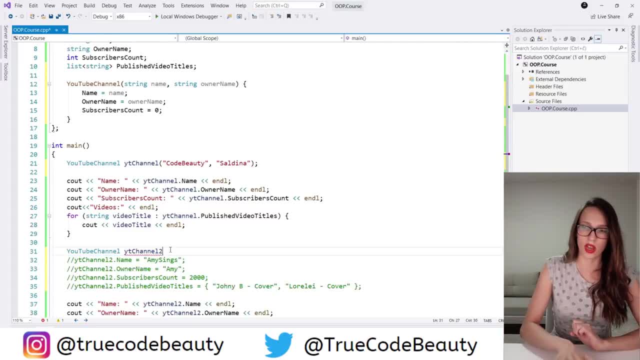 code for a moment, and then here I want to invoke a constructor for this YouTube channel class and pass it as first value- the name, because we are receiving name as our first value in our constructor, like this. And then the second value that we need to pass is going to be owner name. 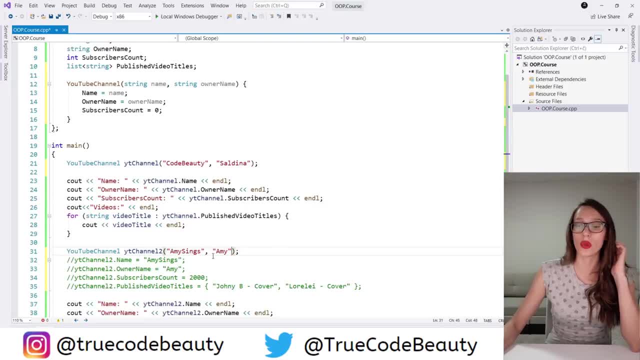 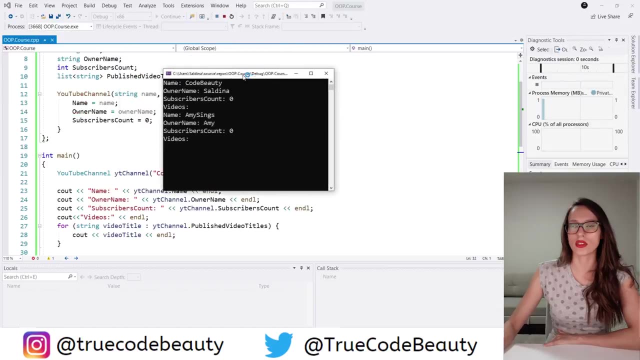 so I'm going to copy that as well. And now we have successfully created this second YouTube channel. Okay, so now I can delete this code here as well. Okay, and now, if I run my program, as you can see, it has written out information about my two 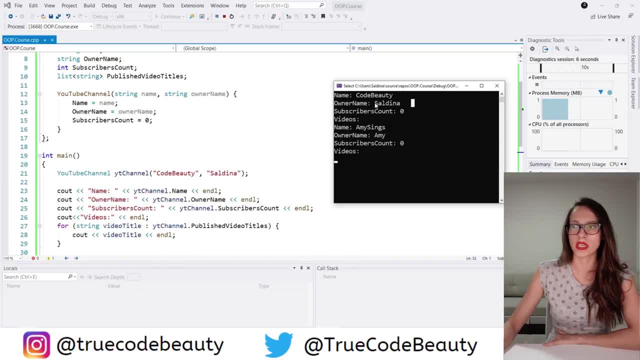 channels. The first one is code beauty. owner is me, and then I have zero subscribers because I have just created my channel and we have assigned that here. And then our second channel is Amy Sinks. owner is Amy and she has written out information about my two channels, So I can. 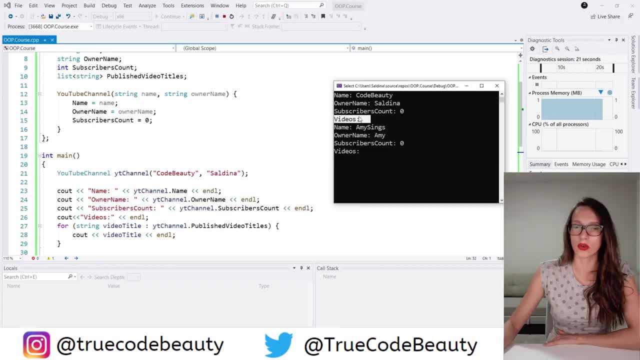 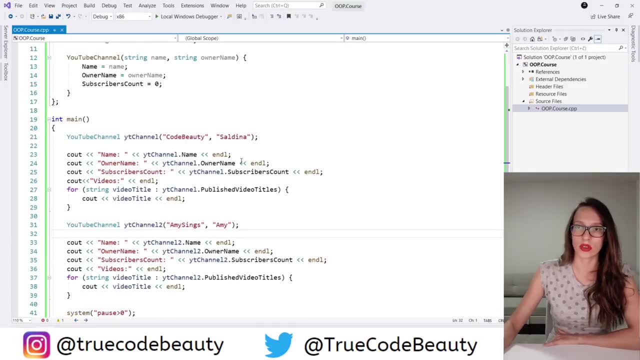 zero subscribers as well And, as you can see, both of these videos published videos lists are empty because we haven't really added any videos. Okay, so how do you do that? I'm going to delete this from here and then move it here, like this, So now we have both of our objects. 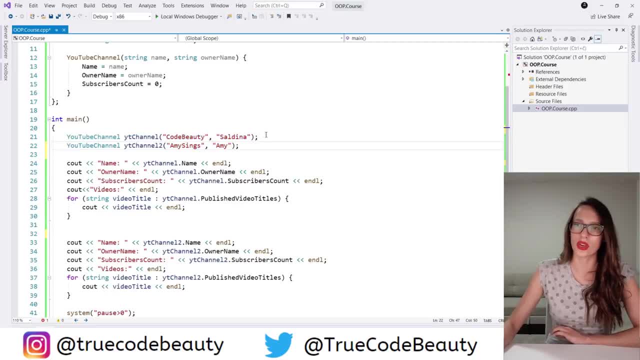 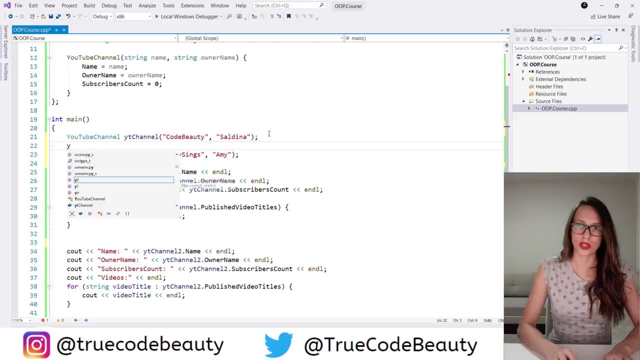 being created at the beginning here. So what I want to do now is I want to add a couple of videos to this channel here. So how do you do that? Well, you say YouTube channel and then you add a couple of videos to this channel here. So how do you do that? 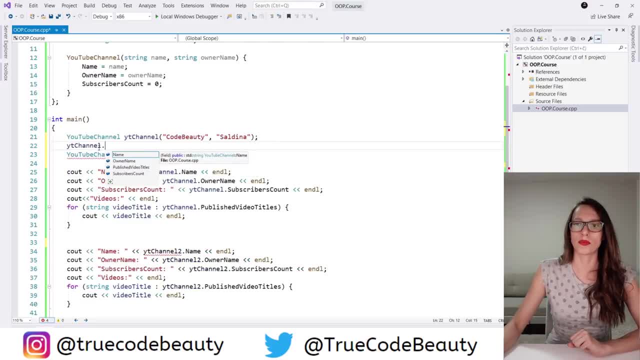 YouTube channel like this, and then I'm going to put dot and here in this published video titles list, I'm going to invoke a method, push back- which is going to add at the end of this list another element, and that element is going to be of type string, because this published video 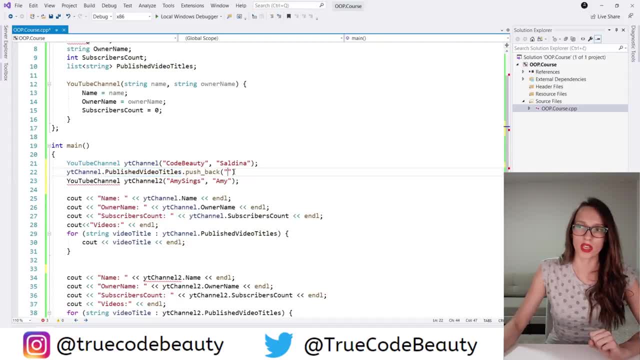 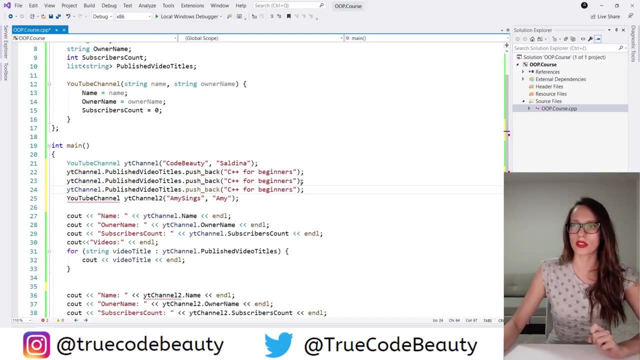 titles is a list of strings. So here I'm going to add a string and I'm going to call that video C++ for beginners like this. So that is one video, and then let's add a couple more videos. 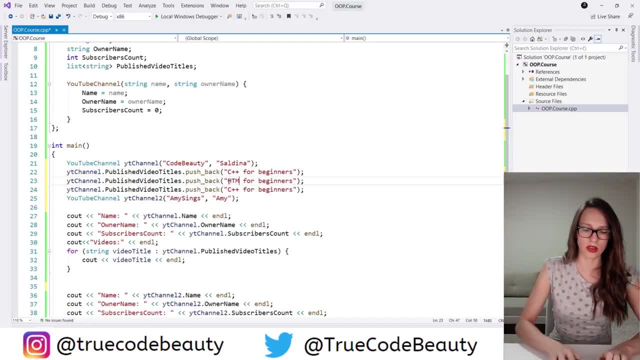 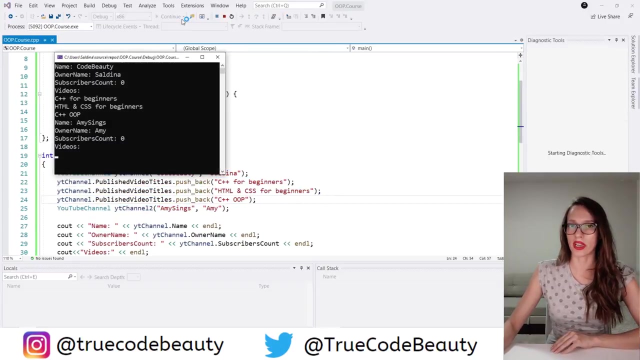 Let's say HTML and CSS for beginners, and then let's say OOP for beginners. Well, no, let's say C++ OOP, like this. Okay, so we have added three videos for this first channel, and then this second channel does not have videos yet. So if I run my program again, you can see that. 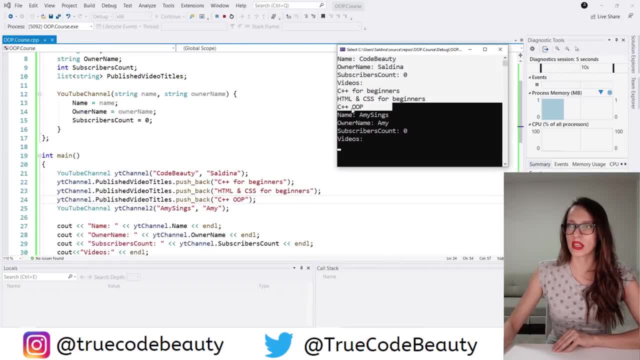 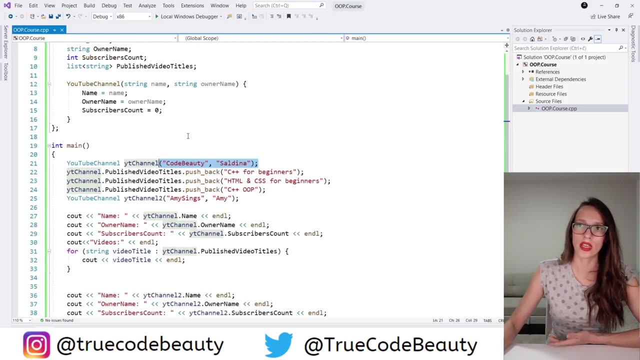 this first channel has three videos, and then this second channel does not have any videos yet, because we have deleted those that we previously had. Okay, now, that was the example on how you can create a constructor and how you can use a constructor, So this here is a. 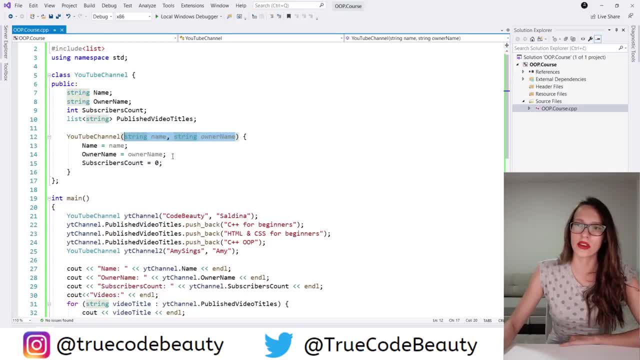 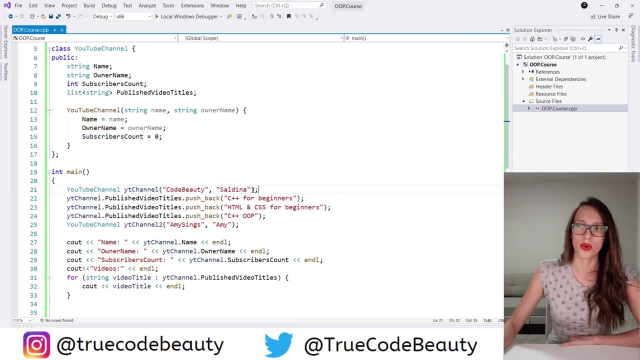 constructor and then here in our constructor we have really assigned initial values to these properties here that we have in our YouTube channel. And then this here is the way that you use your constructor, So you put these parentheses and then you pass the values that. 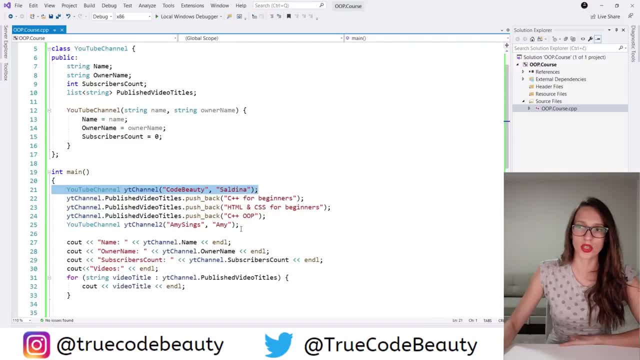 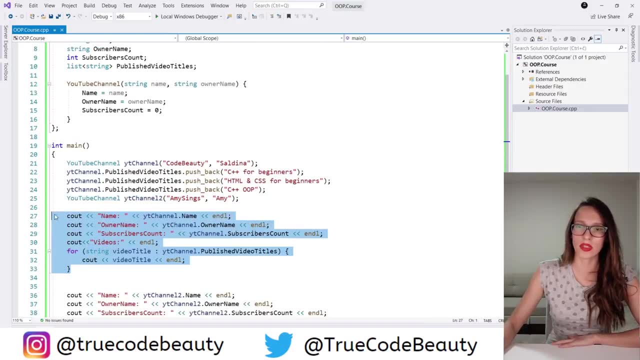 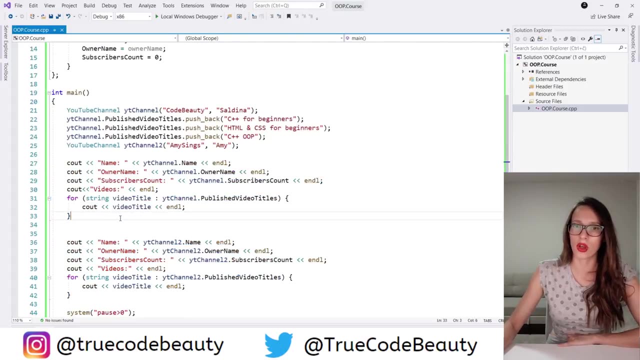 your constructor has to receive, And here we have created two objects, and we have done that without repeating code. Now, what is going to happen with this here? So this here and then this here is repeating code as well, And in order to solve this particular problem, we are going to use class methods. So 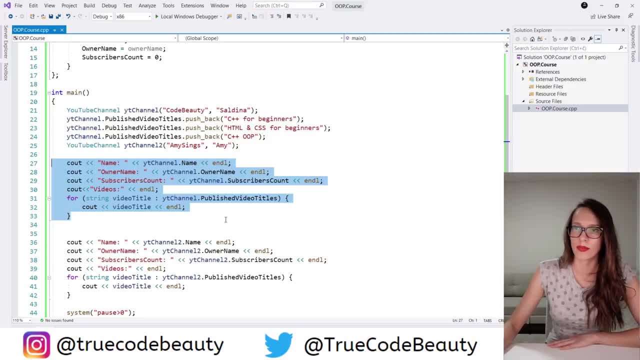 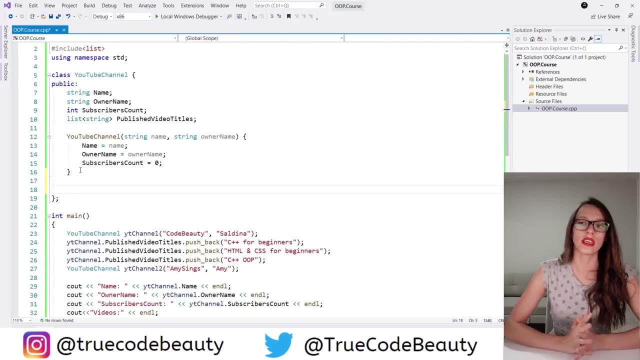 class method is going to describe a behavior of a class, And since here we are writing out these attributes of our class, since we are writing out information about our YouTube channels, what I want to do is I want to create a method that is going to be called getInfo, for example, So that method is going to be of type 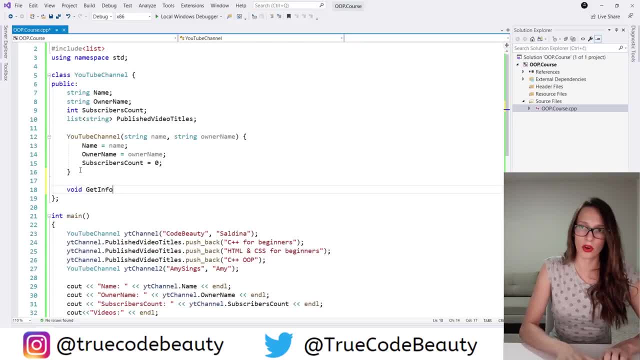 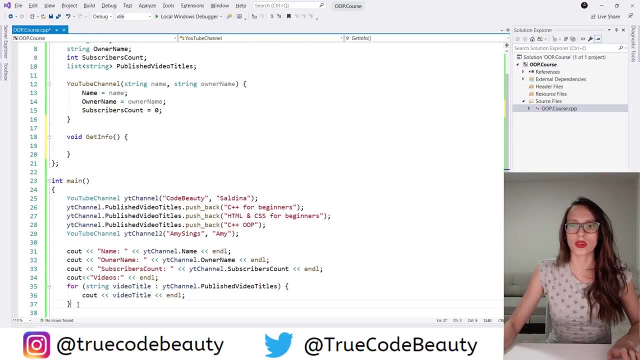 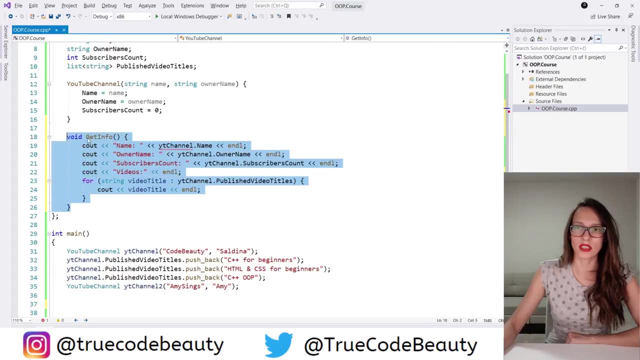 void. Let's call it getInfo, like this. And what I want to do in this particular method is I want to copy this code here, So I'm going to cut it and then paste it here. And in this particular method, in this getInfo, I want to say: please write out name and then the name property. We. 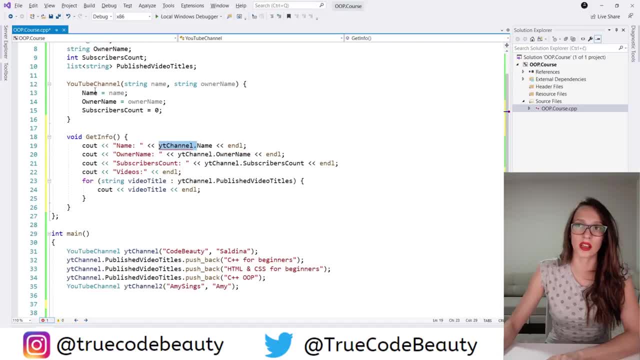 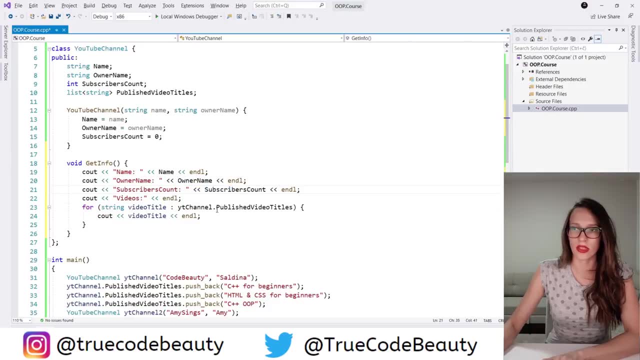 need this YouTube channel object anymore because we are in the class itself. Okay, And then here as well. I'm going to delete this here and then. here And now. this code should work, So whenever you invoke this getInfo method on your object, it should write out all of these properties. 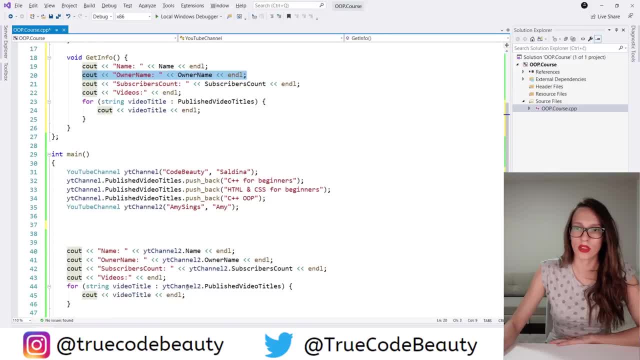 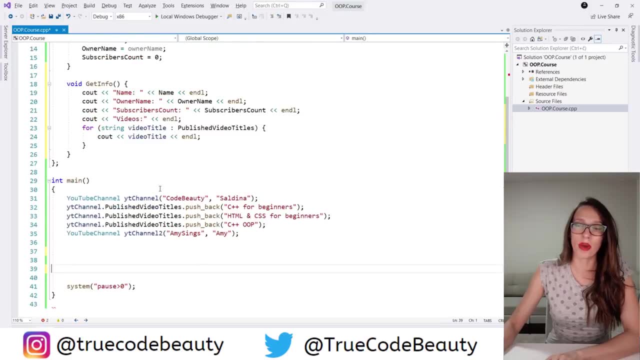 of that object. So now I can remove this code here as well. So this information about our second channel and how am I going to get, how am I going to invoke this method? Well, I say the name of my object, So, for example, YouTube channel, dot, and then, as you can see, I have this. 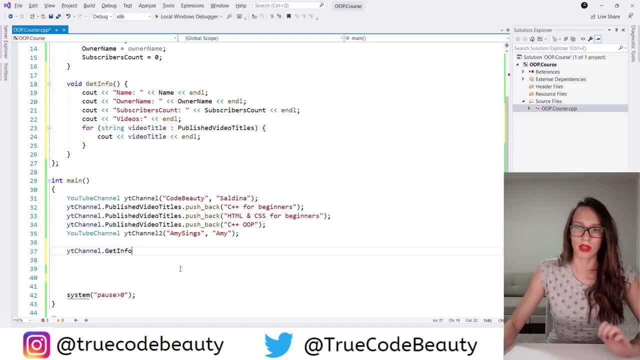 getInfo method available here because it is public. So I say getInfo and I invoke it like I would invoke any other function. And let's do the same for our second YouTube channel. Let's say YouTube channel two: getInfo, GetInfo, like this. And now if I run my program as you can see, it has written out information. 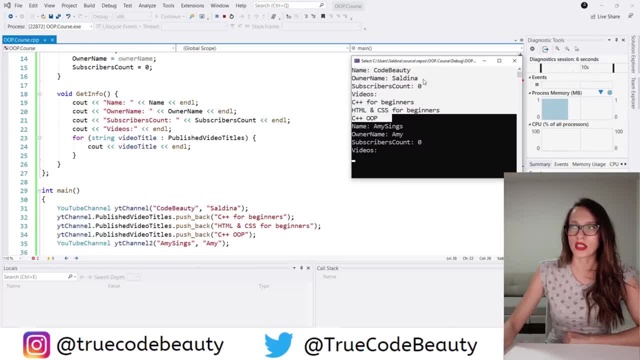 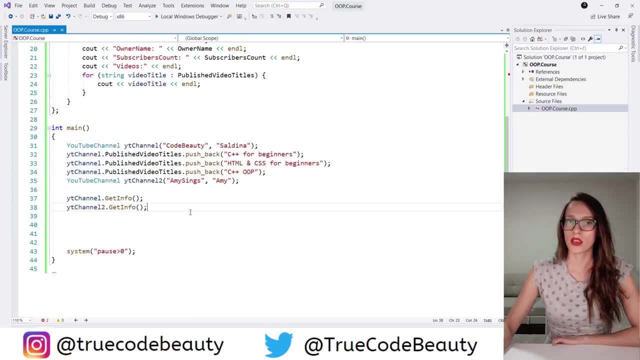 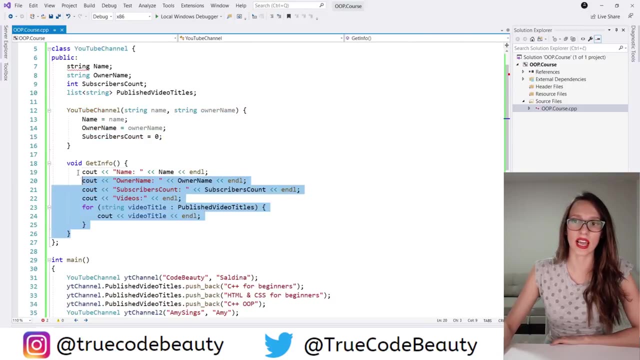 about my two channels. So CodeBeauty Saldina is owner and then subscribers count my videos and then info about my second channel as well. So I hope that you understood the concept behind a constructor of a class and then behind a class method. Here we have demonstrated how you can. 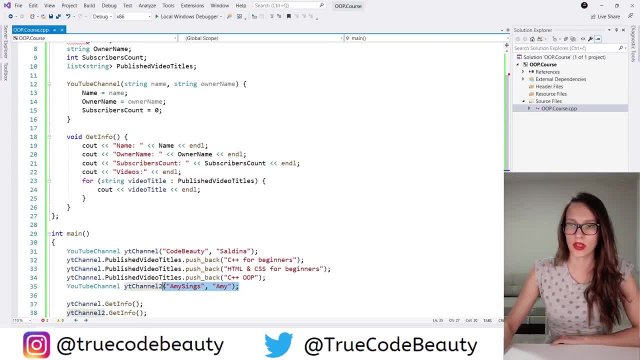 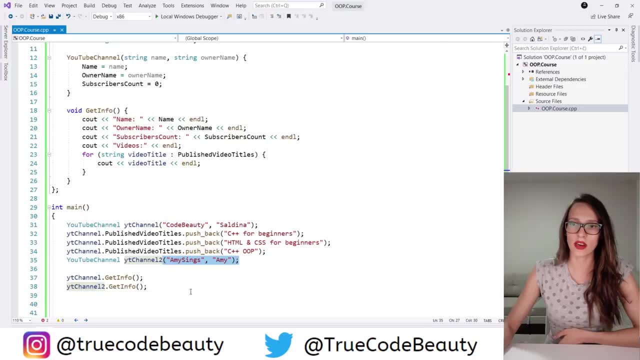 create an object Using a constructor, and then here as well, So you don't really have to repeat your code each time that you create an object. And then here we have invoked a method of these objects which we have implemented here, So you do not have to repeat that code as well Each time that you need to get. 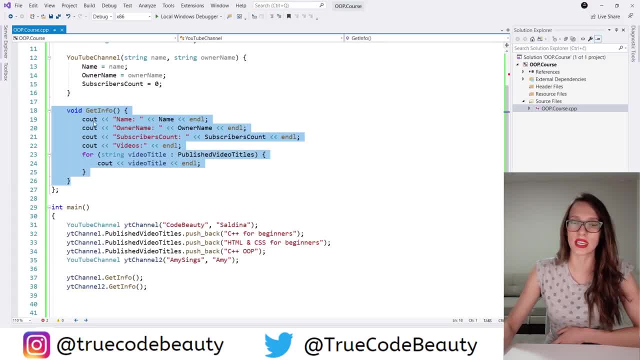 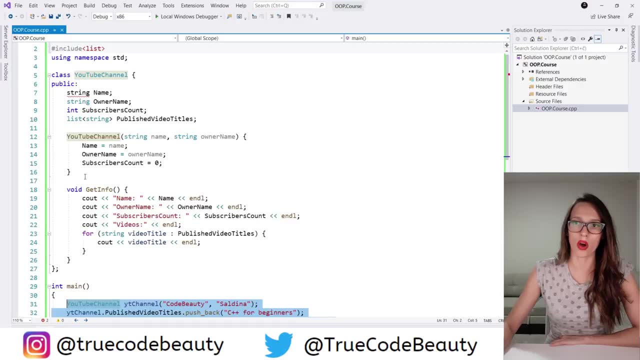 information about your object. you just invoke this getInfo method And now our main function looks much cleaner, and all the implementations of the construction of our objects and then this getInfo method are in this YouTube channel class. So I hope that you enjoyed this video. If you did, give it a thumbs up and also subscribe to my channel. 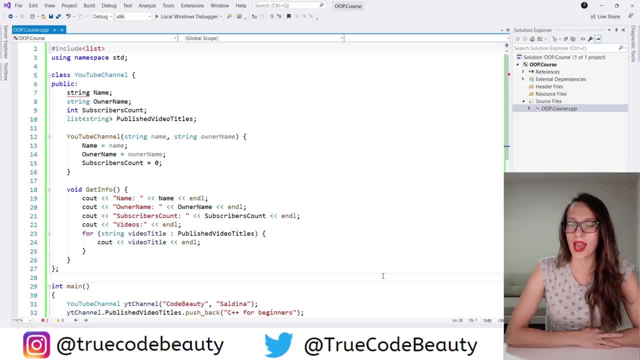 Don't forget to hit that bell icon and I'm going to see you in my next video. Bye.